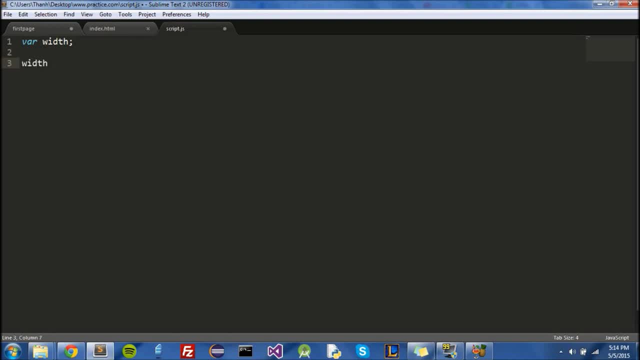 value. So let's give it the width, equals to say five. Let's say, pretend that's like five inches. And let's declare another variable. Let's declare a variable called height, And then let's give this a value of six. Alright, And now that width will have a value of five and height will have a value of six. 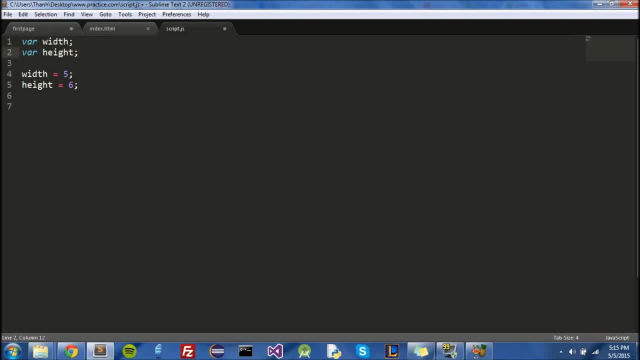 And then when you want to, let's say, calculate the area, you want to make your own calculator- we're going to declare the variable area. And now you could- we're going to go more into this later about assignment operators and the math You can do. let's say, area equals to width, And you're going to use the asterisk, which. 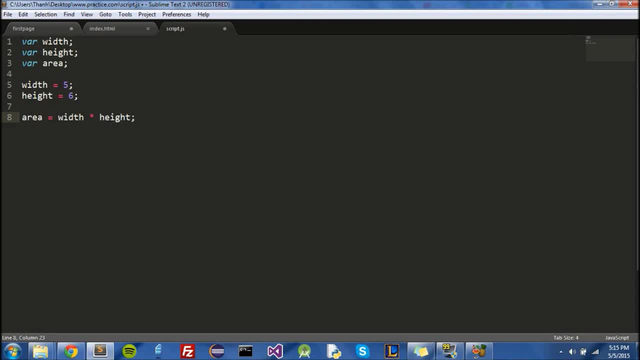 is a multiplication sign, times height, And what this will do is it'll, when the, when the variable is being called within the equation, it's going to take on the value of five, And then, when you call on the height, it's going to take on the value of six And then five. 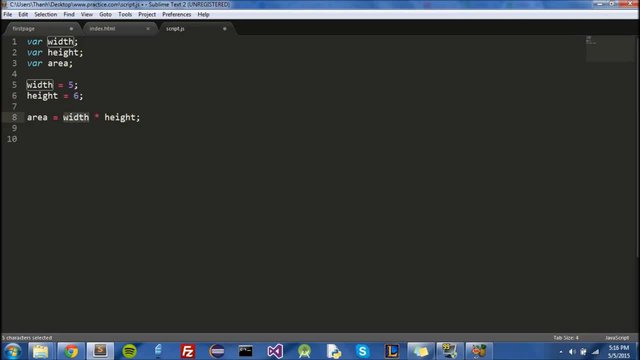 times six is area after this. So that statement is going to be equal to thirty. Alright, And yeah, And let's say you change it before the variable is called in this equation, Let's say width is now equal to ten. This calling to this variable is going to be now. 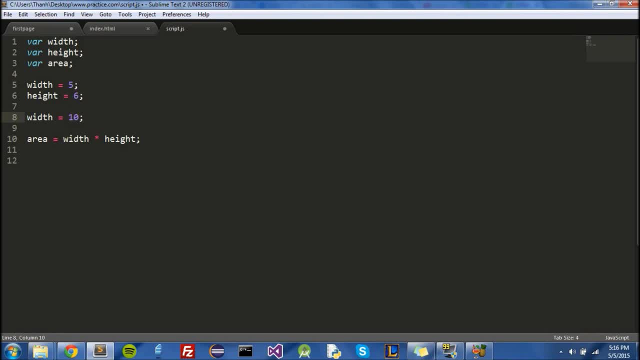 it's going to be ten. It's not going to be five, It's going to be ten because it was the last, the last change. It had the last word in changing the variable, Because it's line 8 and the original one was line 5.. So the line 8 will take dominance over it. 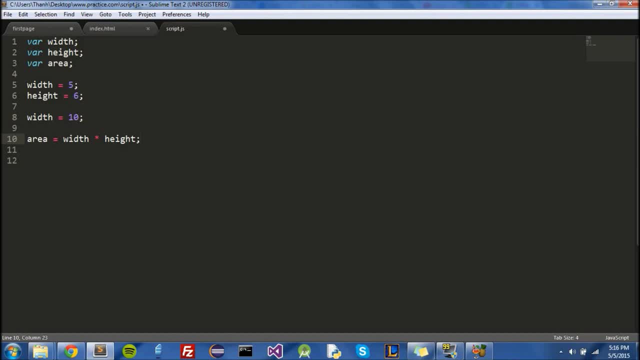 Yeah, let's go over different data types, different types of variables. First there's of course the number, So you can do like var, you can do price equal to 5. That's a number data type, a numeric data type, And variables can also be something. 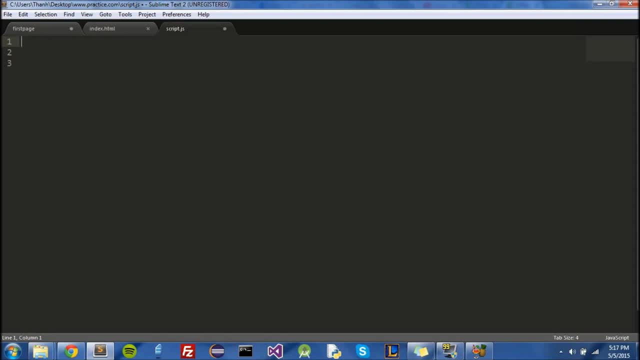 called strings, which are like words And say: var name equals John. This is going to be a string, And strings are always enclosed in either double quotes or single quotes. We'll go over the differences in that later, but either one could be used as of now. 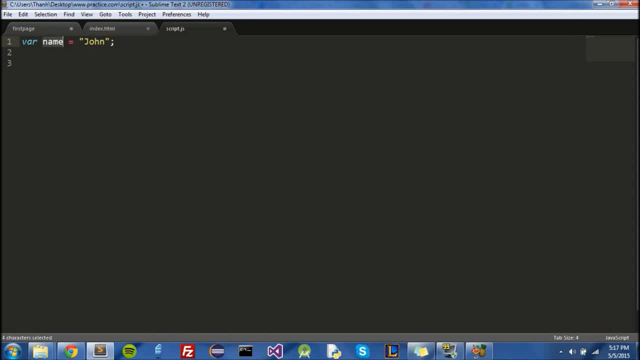 And yeah, when you're going to be manipulating this variable, it's going to spit out a string, And a string is a sequence of different characters. So this is going to be: j separate, o separate, h separate, oh, oops, h separate and n is going to be kind of separate, Like. 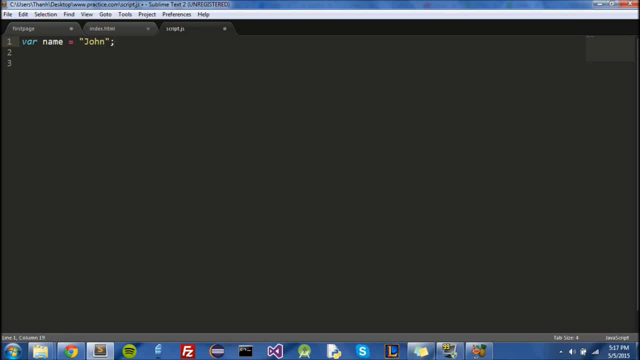 pretend they're in their own separate boxes And when you're calling this variable it's going to bring in these series of characters. Another data data type is called the Boolean data type. Boolean is pretty much either true or false. It has to take one of these values And it's like a type of switch, like a switch in your. 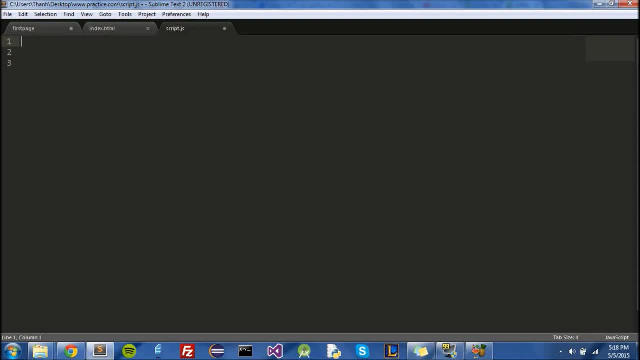 house. Let's say: if the switch is down, it means off and up it's on. So you're pretty much just programming a switch. So let's say var, let's say: Well, that's not a bad example of a switch which is actually important for later. but let's just do button And this: 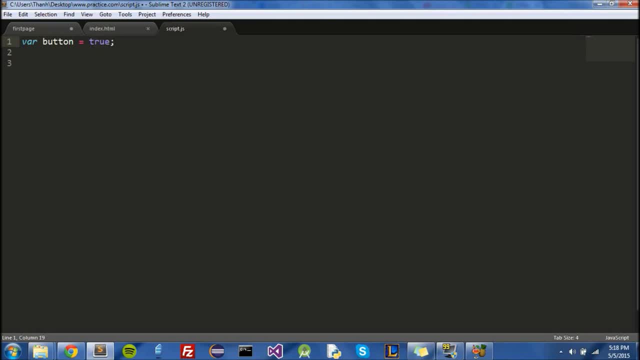 button is going to be equal to true, which is highlighted in blue here. Now let's say for later, if you're testing for a certain condition- say, is it hot outside- and the button variable, if it reads true, then you're going to do a different set of instructions. 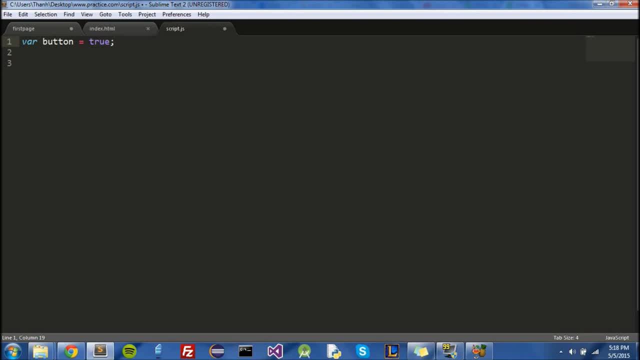 And if it's false, you're going to do another different set of instructions. And yeah, As you see here, this is a Before. I showed you that you declare it first and then you can set it a value later. People, It's up to you. really, Some people, you can. 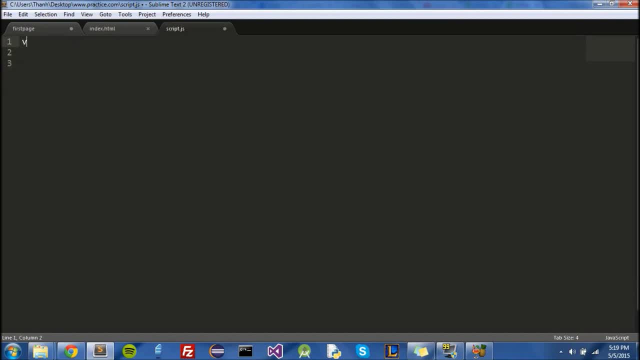 do this, but the shorthand way, of course, is to do the new way I did. it is to just set it in the same line. But sometimes you won't have a value for it at that point in the program, so you're going to want to set it later. Let's say that it hasn't been set. 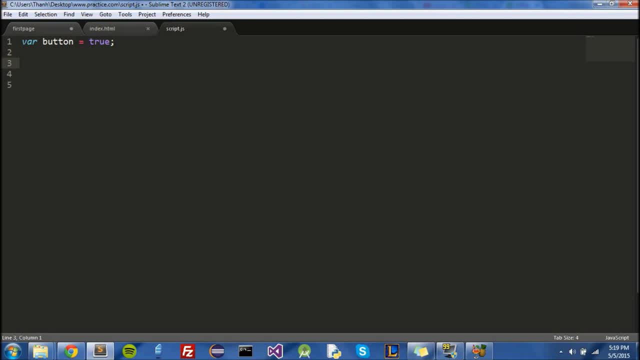 yet and you need to calculate something before the variable is actually set. Let's say, like the area in the previous example, because the area wasn't really set until height and width were multiplied by each other. And yeah, And let's go over some rules of variables. A variable, first rule, it must begin with. 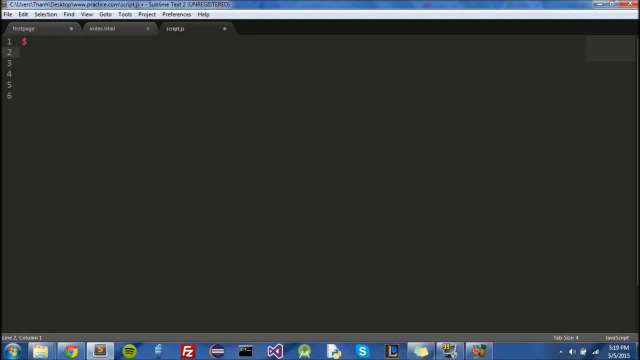 either a dollar sign, A underscore or a letter Like A, B, C, D, E, F, G. you know the alphabet And rule number two: it can contain letters, dollars or an underscore, but you can't use like. 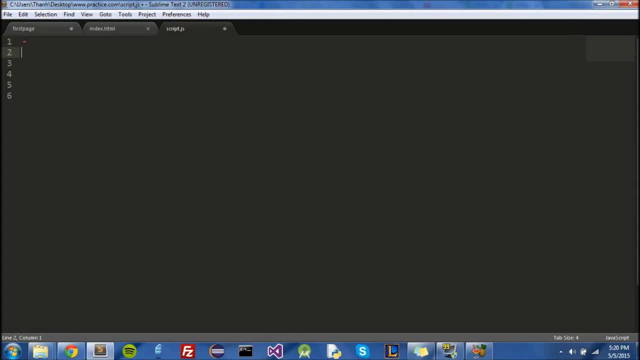 dashes or like or periods. Um, The usual convention of variables is that usually if you have multiple words in a variable- let's say like dark alley- this is called a camel casing. The second word in the variable name is usually capitalized and the first word is usually always lowercase. So you can. 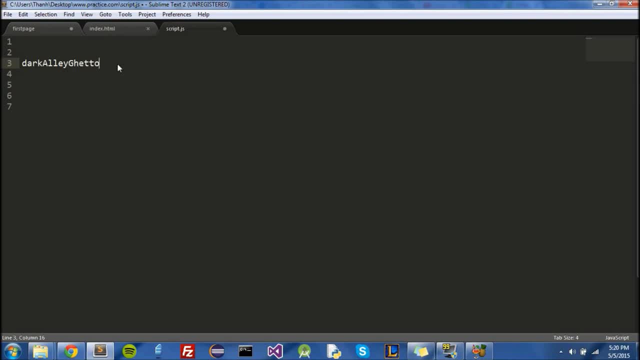 have dark alley, ghetto and all the following words will have to have a. well, not have to, but it's usually a convention. It's a good thing to get in the habit of: Um, Uh, yeah, Uh, rule number three: um, you can't use, like reserved keywords, Like you can't use. 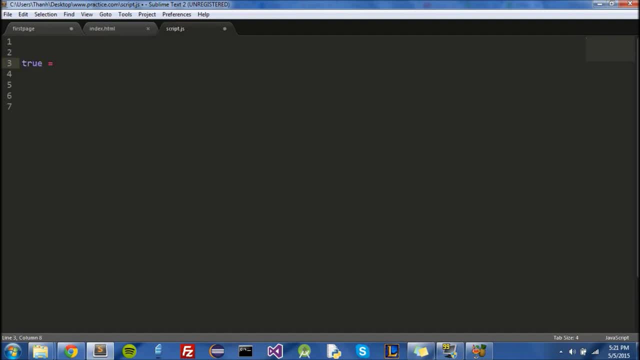 like true, because you know, uh, true is reserved for belay and ballot variables. And like switch, like remember we were trying to use switch, but that was a bad example, because switch is used, it's reserved for a different, uh, a different part of its. 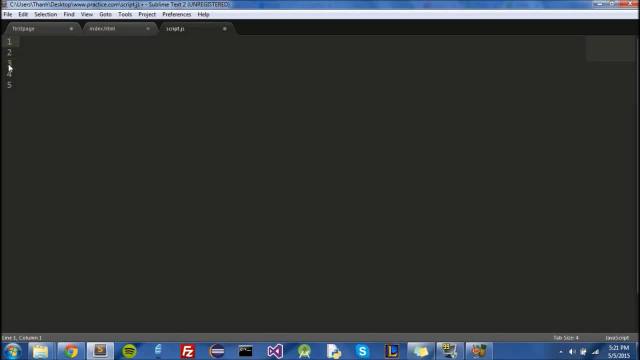 uh program, a different part of the JavaScript uh programming language. Uh, yeah, And uh, rule number four: Um, JavaScript Rules for variables are case sensitive, so score is going to be different from score. Um, these are both fine, oops, changed. These are both fine variables, but um, if you're.